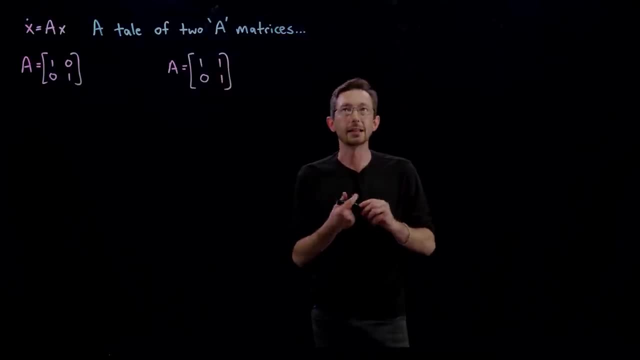 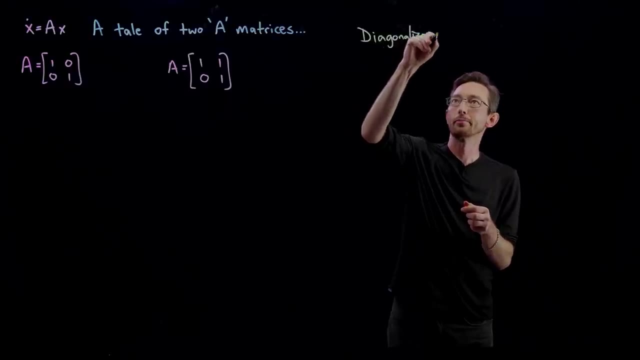 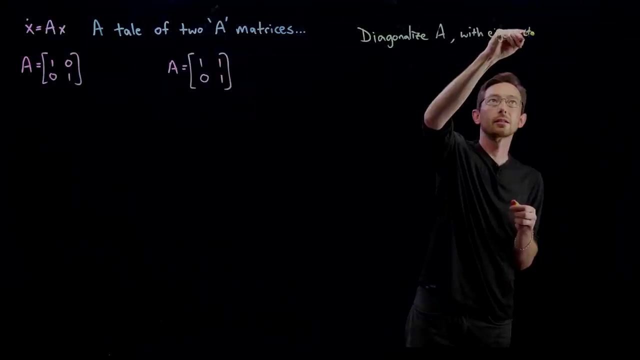 So in the cases I've shown you in the past, there is essentially this idea that you can diagonalize A with eigenvalues and eigenvectors, Diagonalize A with eigenvectors and eigenvalues, eigenvectors and eigenvalues, eigenvectors and eigenvalues, And specifically my eigenvectors. 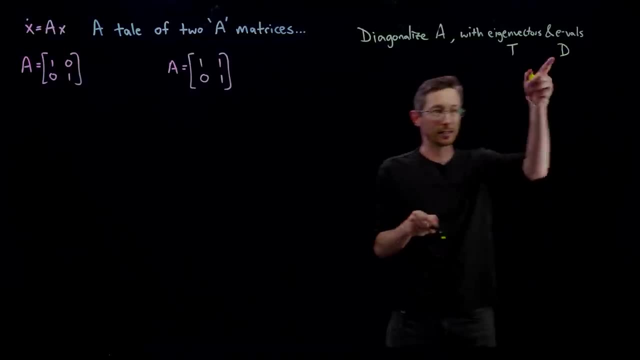 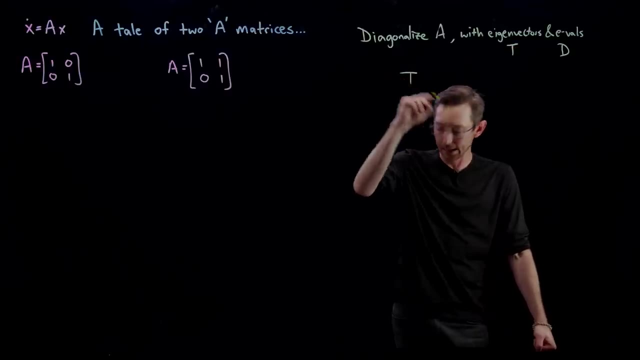 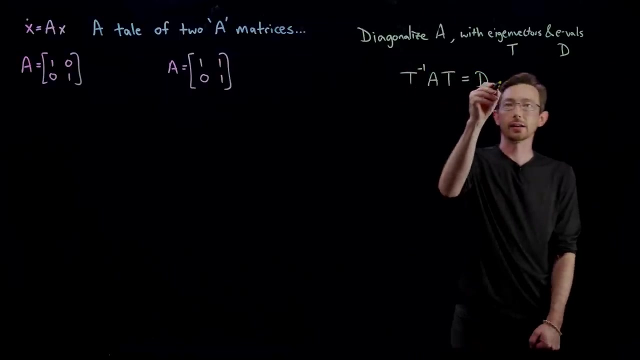 come in a matrix T and my eigenvalues come in a diagonal matrix D, And if I have a matrix that has these eigenvectors and eigenvalues, then I can take T, inverse A, T and that's going to equal this diagonal matrix And what we've been assuming up until now is that this diagonal 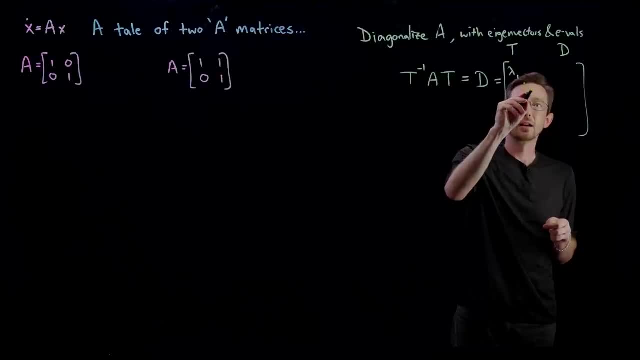 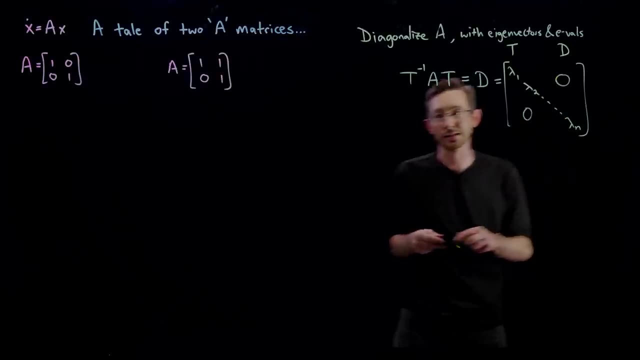 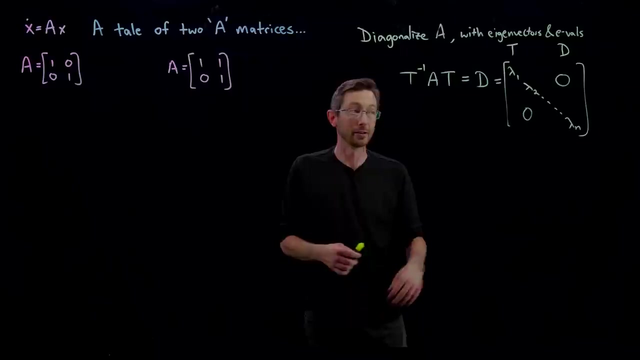 matrix essentially consists of lambda 1, maybe I'll write lambda 2,, dot, dot, dot, lambda N and zeros. everywhere else I've been kind of implicitly assuming that all of these lambdas are distinct and different eigenvalues, not like this case where I have repeated. 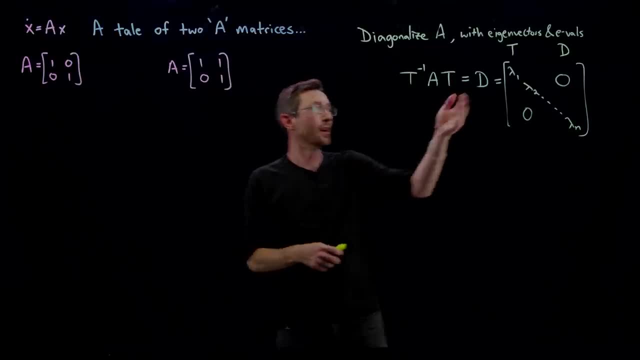 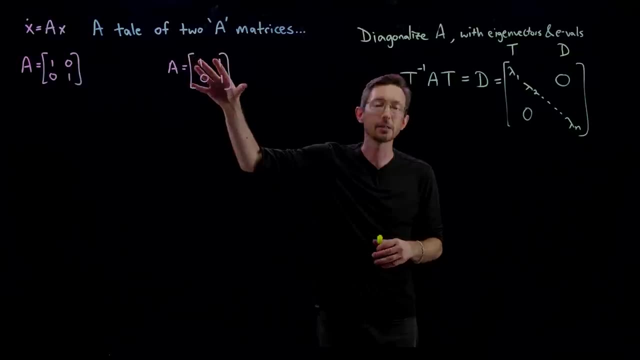 eigenvalues, where I have two eigenvalues that are lambda equals 1. I've been kind of implicitly assuming that I have distinct eigenvalues here, And so this is a little bit of a special case I'll tell you about, and then we'll revisit this kind of general diagonalization here. 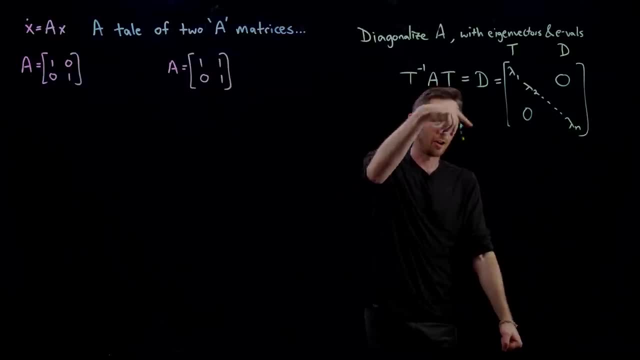 And so, specifically, there are some kind of math theorems. I don't usually give you like theorems and proofs and like real kind of things, but I'm going to give you some kind of rigorous math. I give you just the feeling of the math, But there's some important properties. 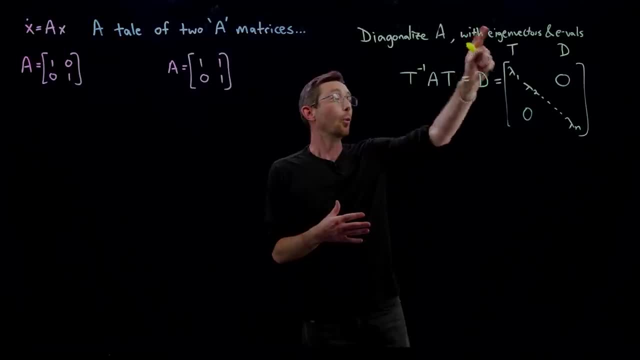 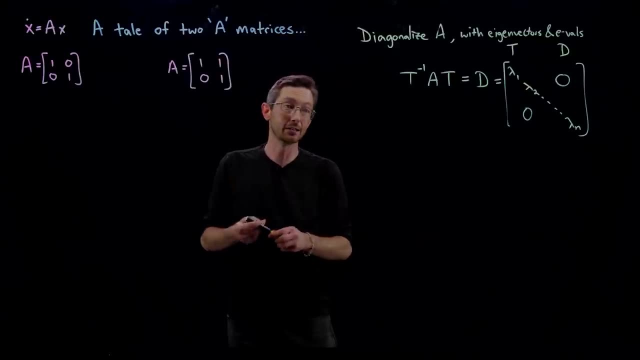 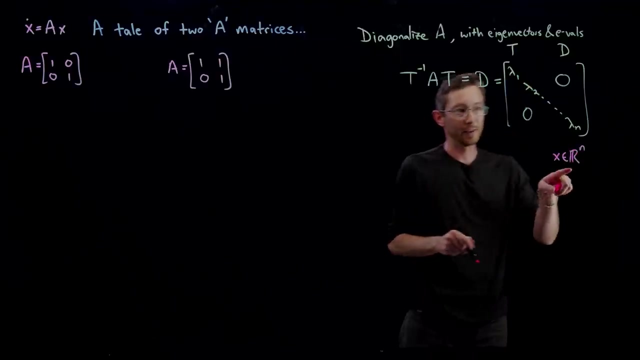 of when you can diagonalize a system like this, when the eigenvectors T form a complete basis for this N-dimensional vector space that my vector X lives in. So you know X lives in an N-dimensional vector space. This means it's an N-tuple of real numbers, It's a vector, okay. 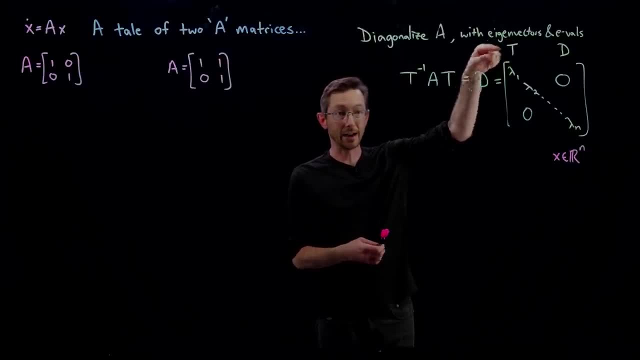 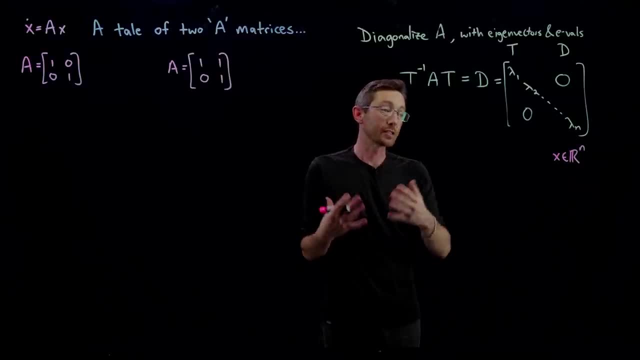 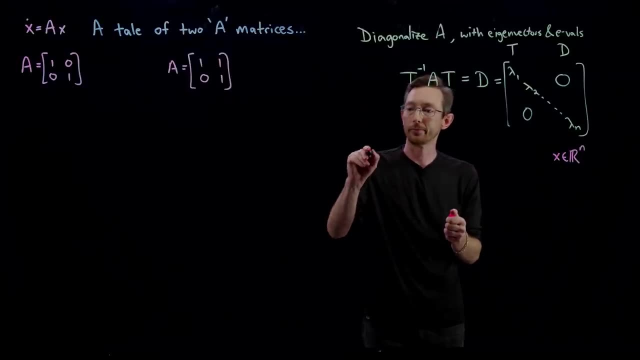 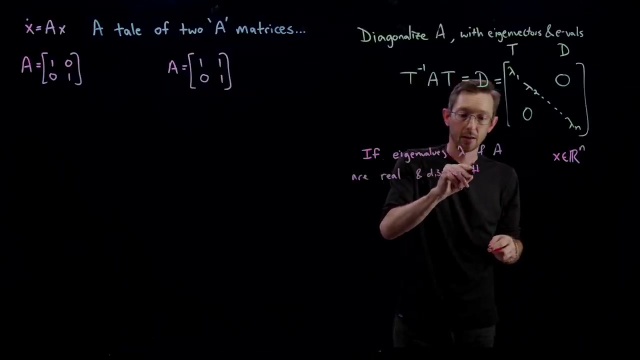 all of those eigenvectors, all of those directions will span a basis for this N-dimensional vector space. if so, if, if all eigenvalues, if all the eigenvalues lambda of A are real and distinct- real and distinct meaning they're not equal to each other- then essentially, my eigenvectors T, the eigenvectors, 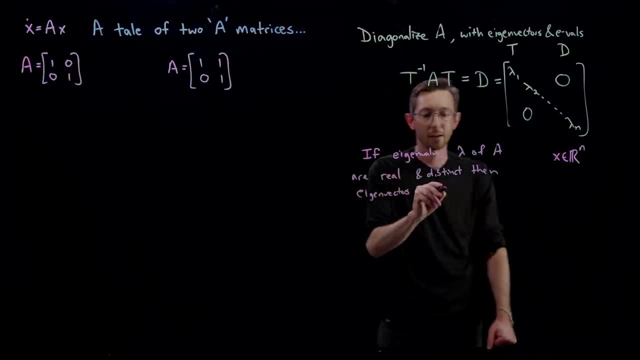 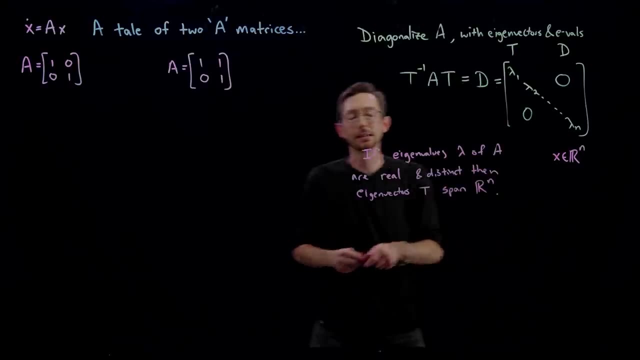 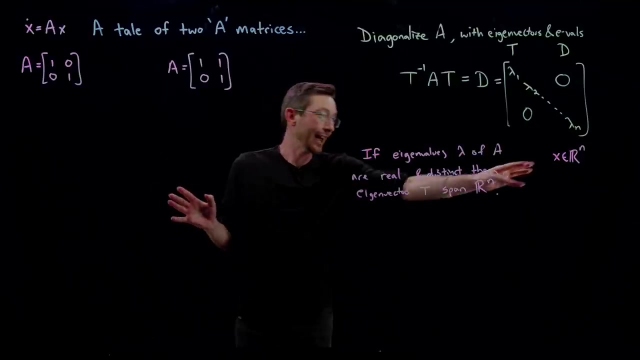 eigenvectors T span this N-dimensional vector space. They span Rn And what that means is this is a real N-dimensional vector space. What that means is that any vector you could name, any X in this space that you could possibly name- is going to be a linear combination. 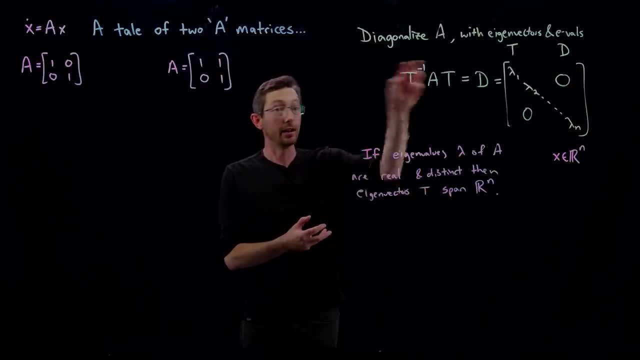 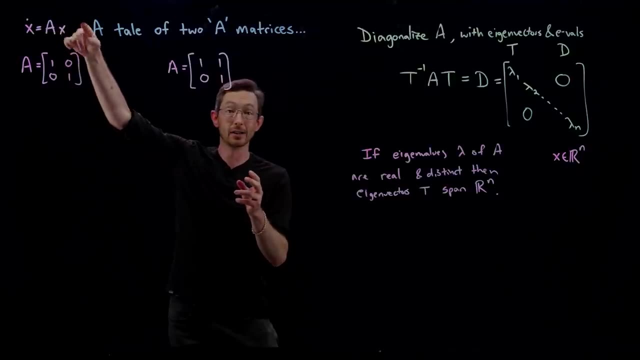 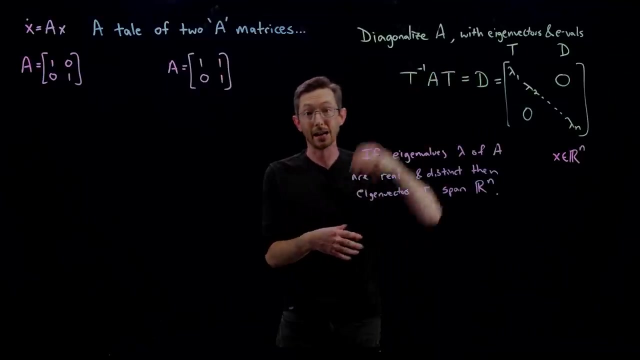 of the columns of T or of the eigenvectors of my A matrix, And that's a really useful property. That means that kind of any initial condition I have, any initial state, any X vector in this space can be written as a linear combination of columns of my eigenvectors, the columns of the matrix T. 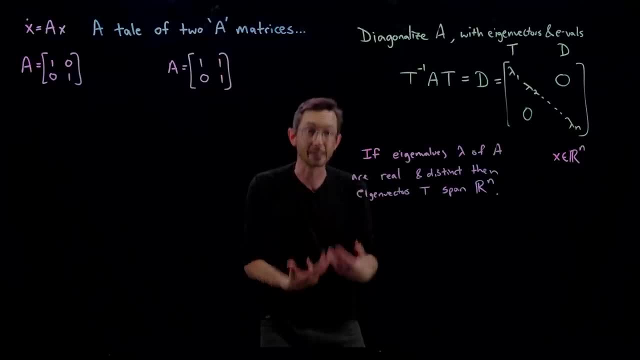 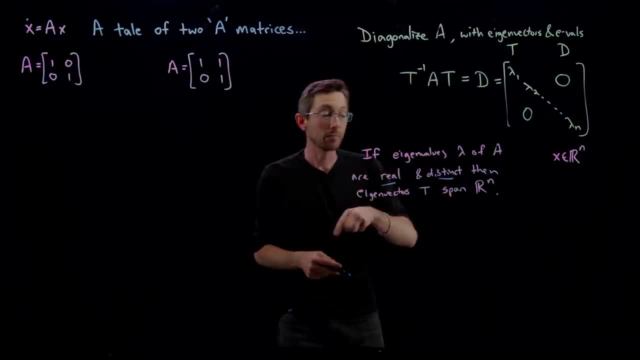 So I'll underscore real and distinct. If they are not real or they are not distinct, then there might be some issues with this diagonalization procedure. I won't be able to write it as a purely diagonal system. There might be a couple of off-diagonal entries, like this guy. 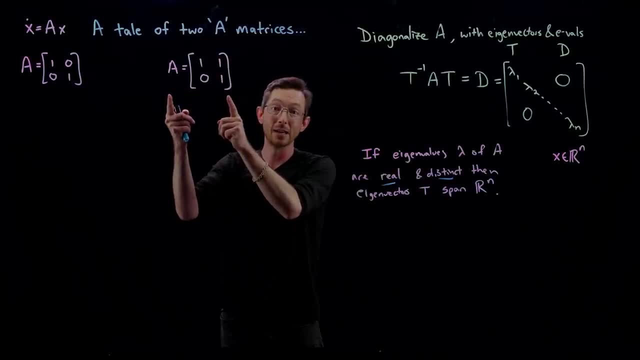 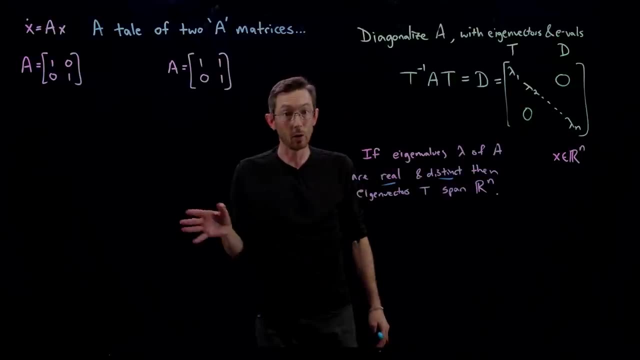 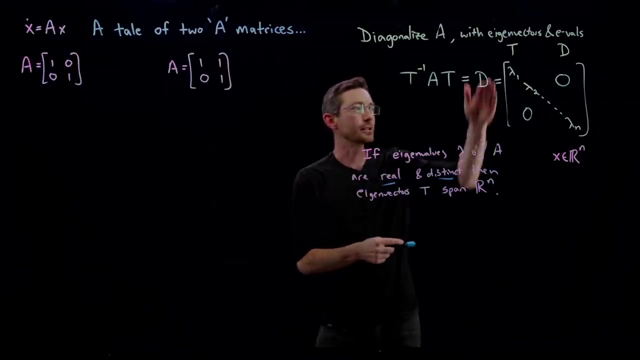 here. It's impossible to perfectly diagonalize this matrix. I'm always going to have this off-diagonal entry here in my D matrix, no matter what I do. There's no coordinate transformation that will get rid of this. I'm going to have this little upper one that's not diagonal, And so there's exceptions to this idea. 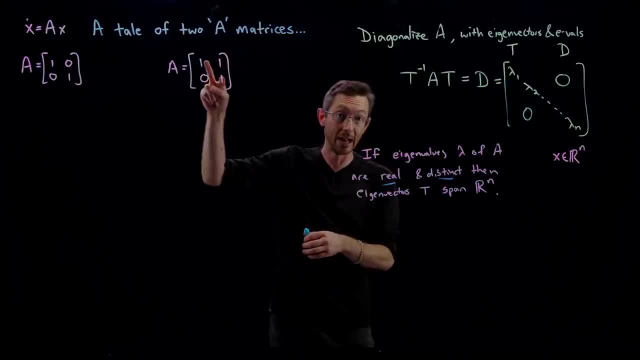 that you can diagonalize your matrix, In particular if I have repeated eigenvalues, sometimes I won't be able to get perfectly diagonal matrices, But you get things that are close to diagonal And I'll show you that kind of in this lecture. Good, So we'll revisit this in a little bit. 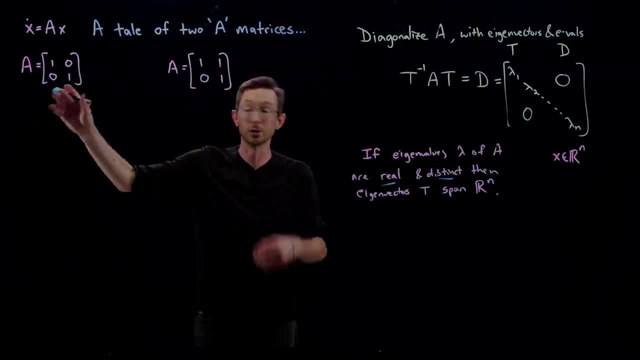 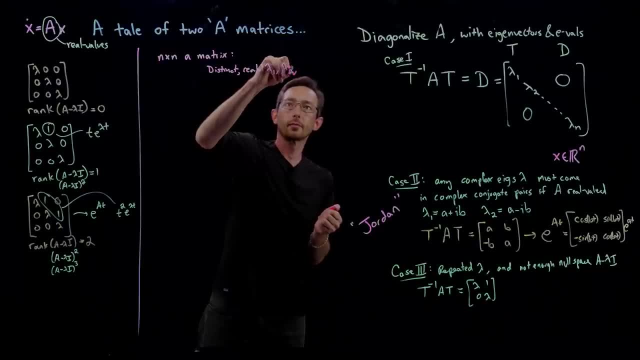 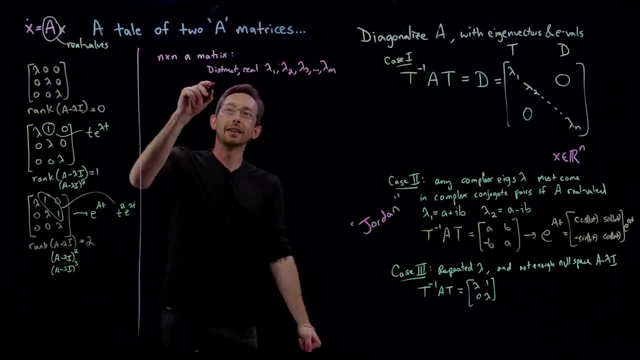 So clearly this matrix is not going to be a diagonal matrix. So clearly this matrix is not going to be a diagonal matrix. Lambda3 dot. dot to Lambda M. I've got M distinct eigenvalues. And then also, let's say, I have complex conjugate pair. 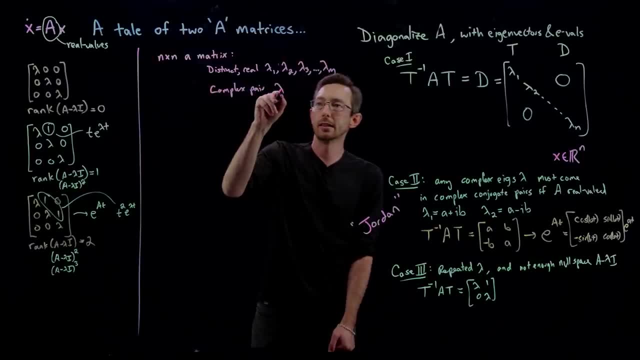 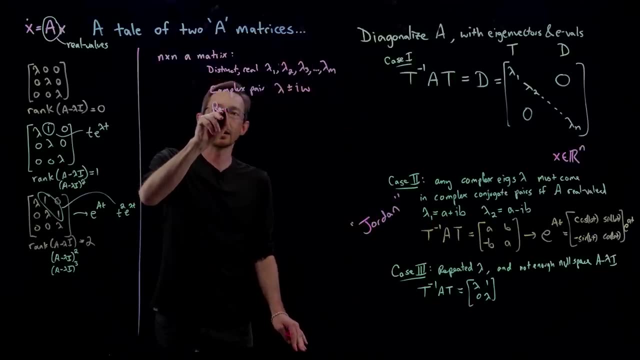 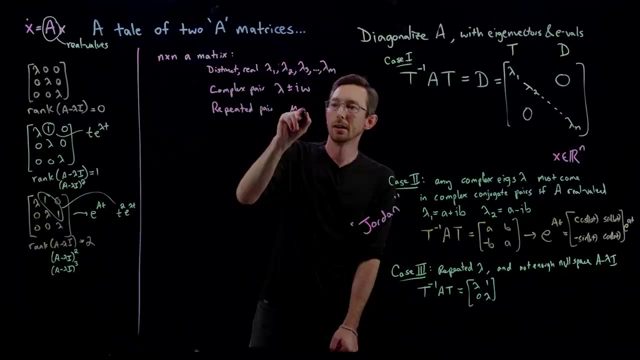 Complex pair. Let's call this: Lambda. plus or minus i, omega, That's a complex conjugate pair. And then let's say: I have a repeated pair, Repeated pair and let's give it a different name. let's call it, you know, mu times two. I've got two muse, but a minus mu. I has a 2d. 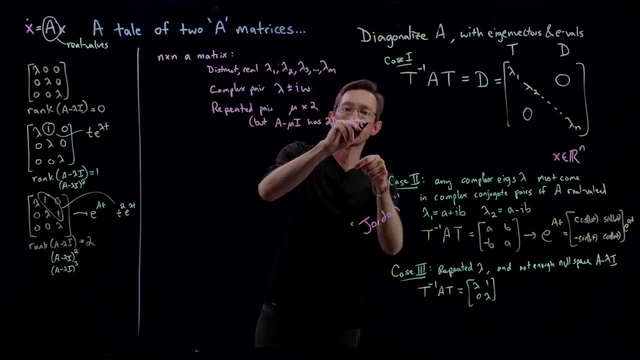 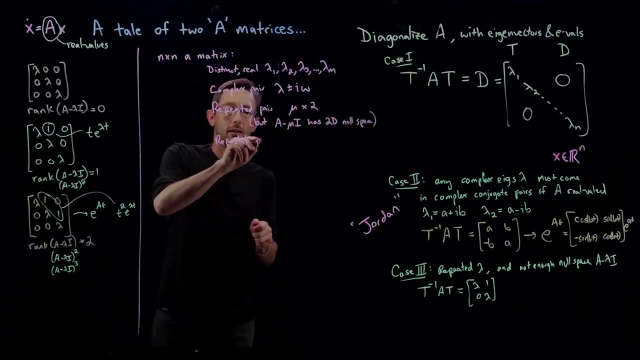 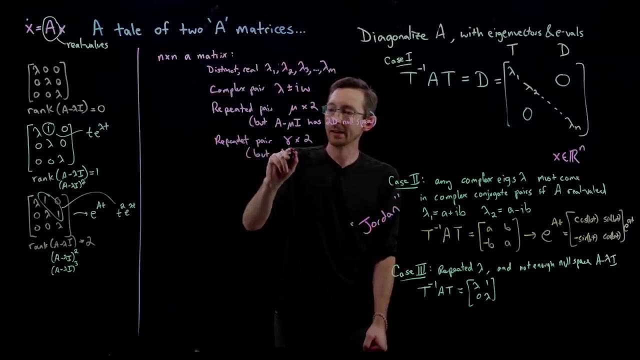 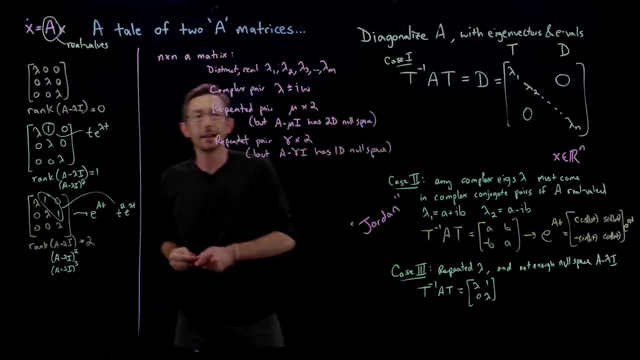 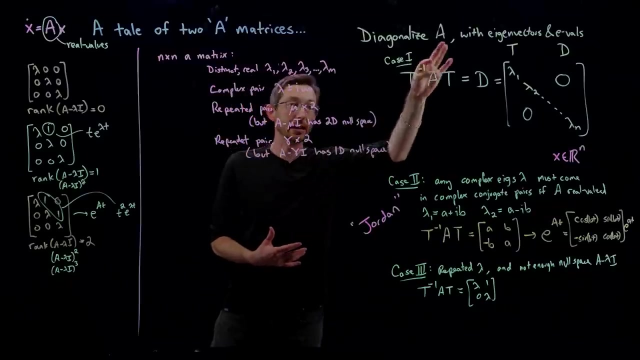 null space. and then, finally, let's say I have a repeated pair. repeated pair instead of mu, let's call it gamma times two, but a minus gamma. I has a one dimensional null space. then, by finding all of the eigenvectors corresponding to all of these eigenvalues, I can transform my system with T inverse a T into what? 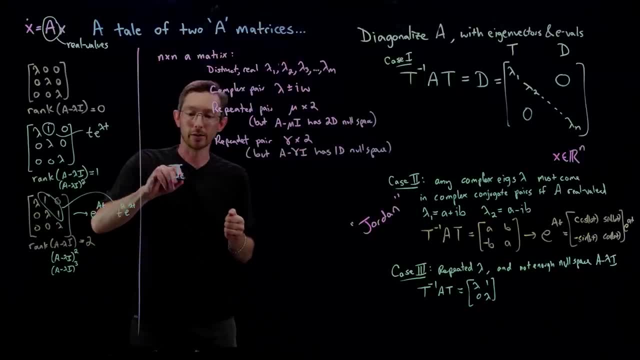 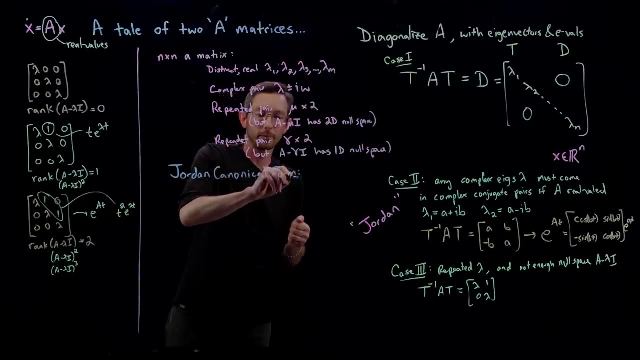 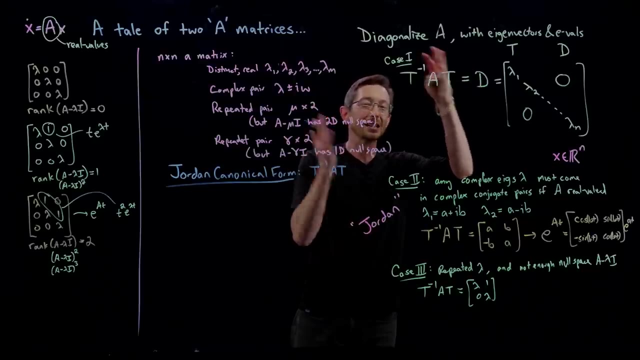 is called the Jordan canonical form. so the Jordan canonical form, canonical form that I would get by taking T inverse a T, it's not going to be strictly diagonal but it's going to be as close to diagonal as you can get for this system and so that Jordan form it's going to have a big block, that is. 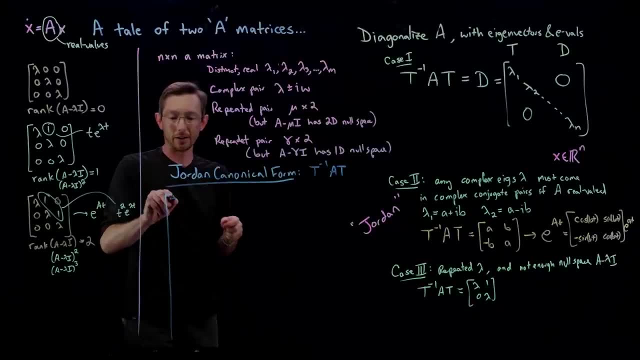 diagonal. so it's going to be this huge matrix and it's going to have, you know, lambda 1, lambda 2, dot, dot, dot to lambda M, zeros here. so this is a block matrix that's diagonal. so this is a block matrix that's diagonal. so this is a block matrix that's diagonal. and then I'm going to have 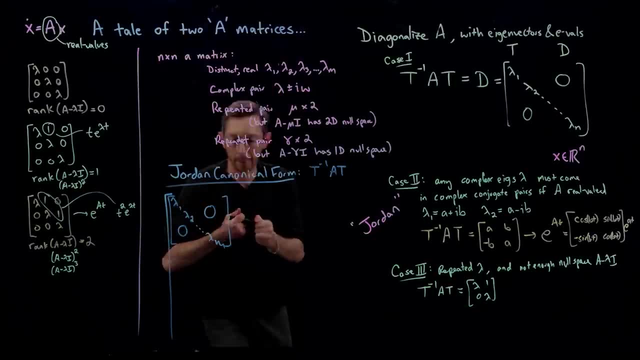 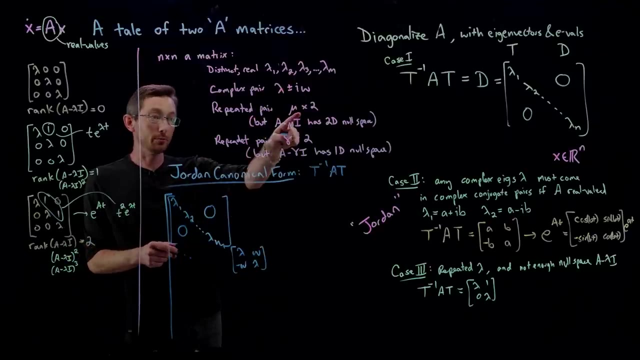 and then I'm going to have another Jordan block below it for this complex pair. so I'm gonna have this little block here which is, I believe, lambda, Omega minus Omega lambda, this little Jordan block there, and then I'm going to have another Jordan block for my repeated eigenvalues, but because a minus mu I has. 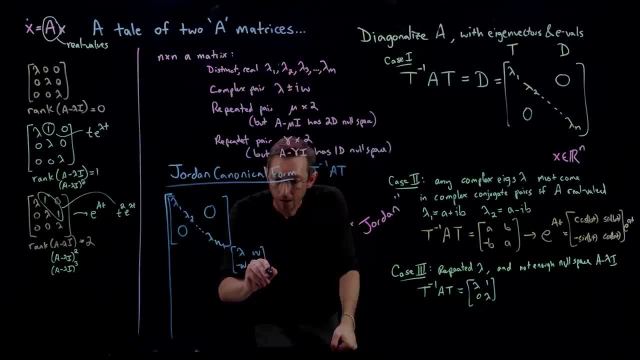 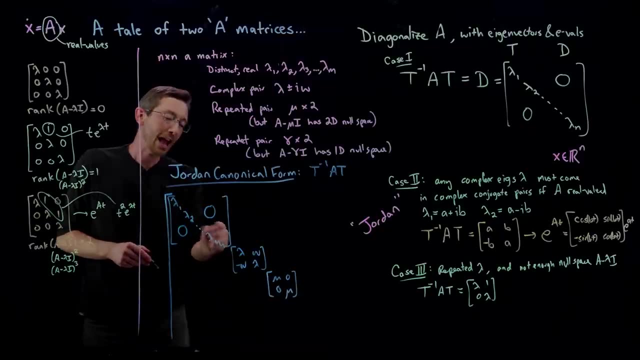 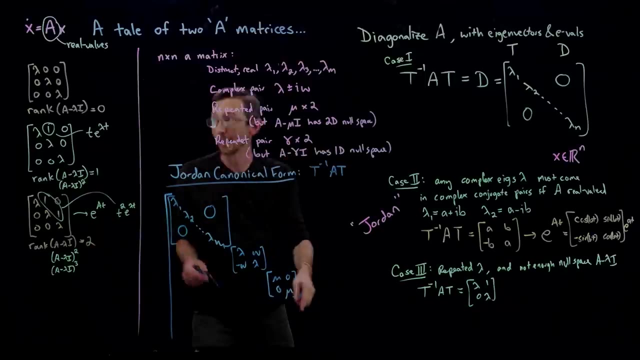 a two-dimensional null space. I can diagonalize this one, so I'm gonna have a little mu zero, zero mu block. it'll actually be diagonal. and then my final block for these eigenvalues, the Jordan block for this, because a minus gamma i only has a one-dimensional null space. 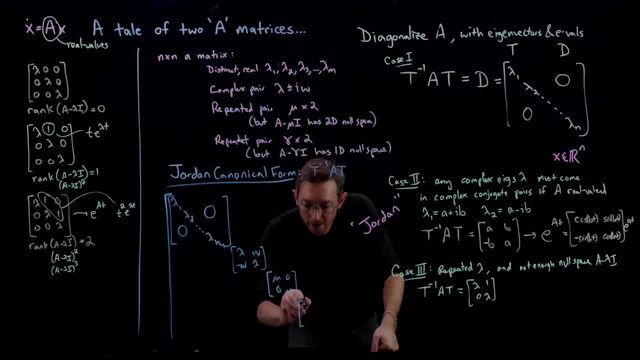 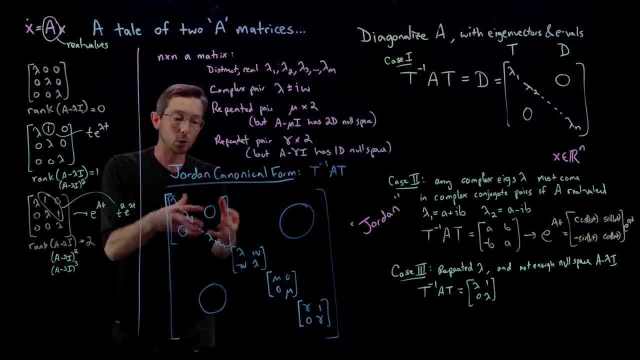 it's going to look like this and that Jordan block is going to be gamma, one zero gamma and everywhere else is going to be zeros. so this is as close to diagonal as possible, but it's block diagonal in terms of these Jordan blocks. so my real and distinct eigenvalues actually form a. 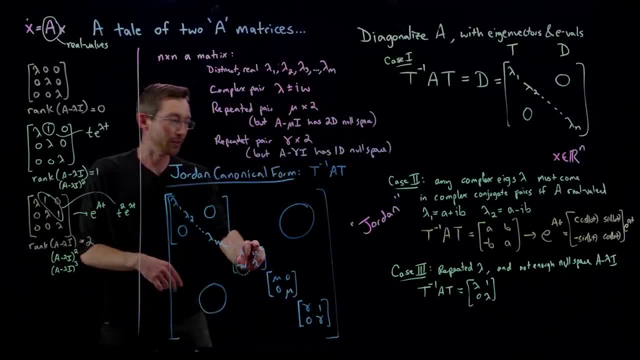 diagonal Jordan block, my complex conjugate pair, form a kind of skew symmetric block. my repeated pairs that have a big null space are again diagonalizable and my repeated pairs that have a rank deficient null space have this extra secular term here and so every single system that is. 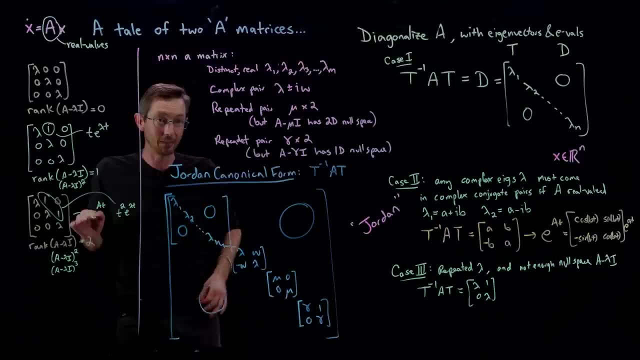 n-dimensional, every single real valued, a matrix you could possibly name. you can find it in the description of this video and I'll see you in the next video: eigenvalues: you can look at the ranks of the null spaces and you can write through an eigenvector. 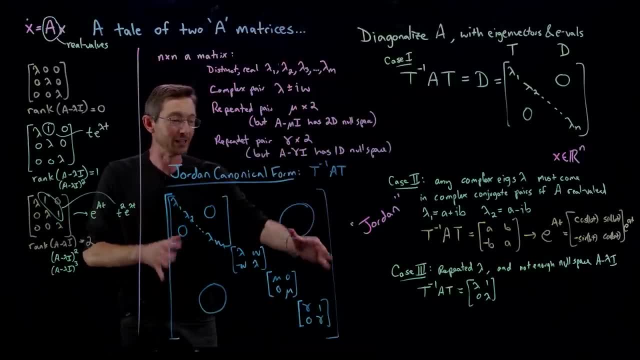 change of coordinates that system into this Jordan canonical form. this is kind of like the universal decoder ring for all linear systems, all a, and if a single one of these eigenvalues has positive real part, it's an unstable system. if all of these eigenvalues have negative real part or zero real, 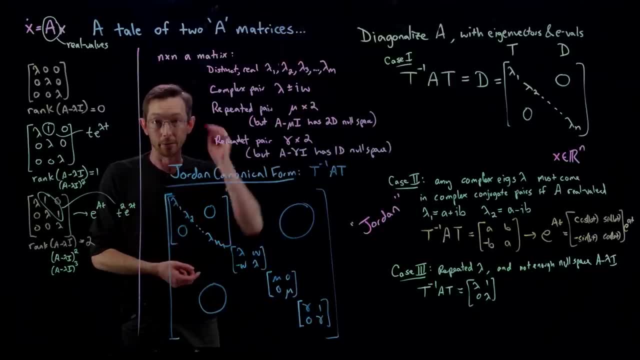 part. then it's either asymptotically stable or neutrally stable. okay, really cool stuff you can do. okay, that was a lot, that was okay, but this is important. this is one of the coolest things in linear systems is kind of getting to this Jordan form. this is really an important concept. so I'm glad you got to see it all right, thank you. 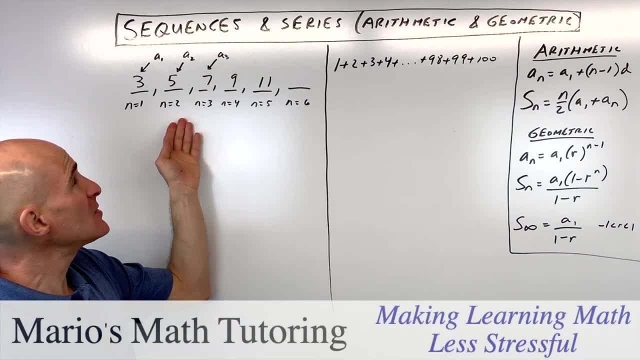 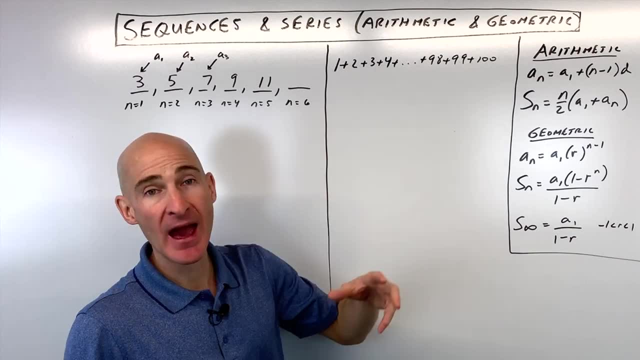 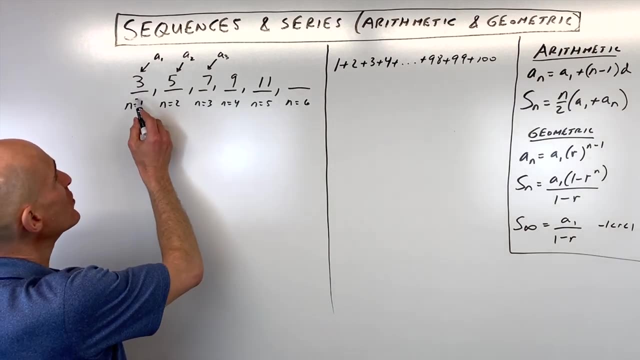 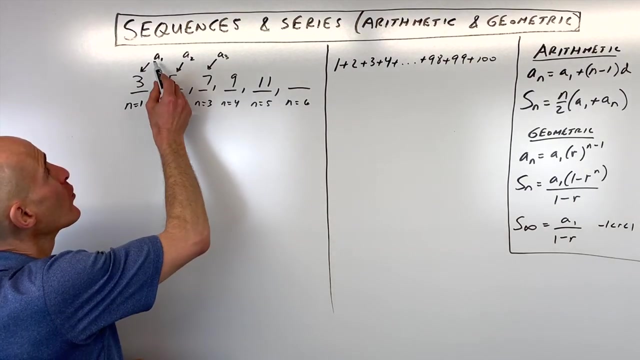 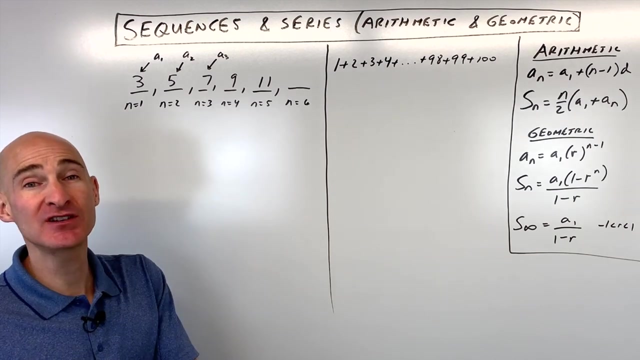 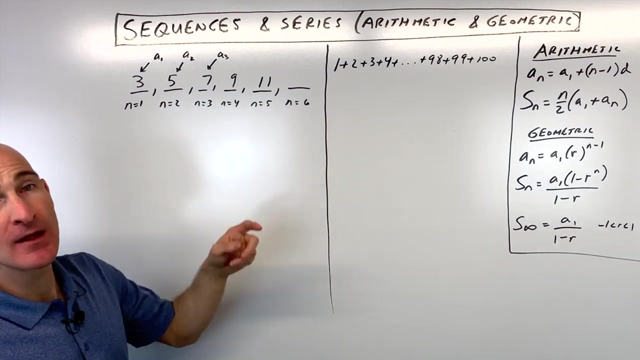 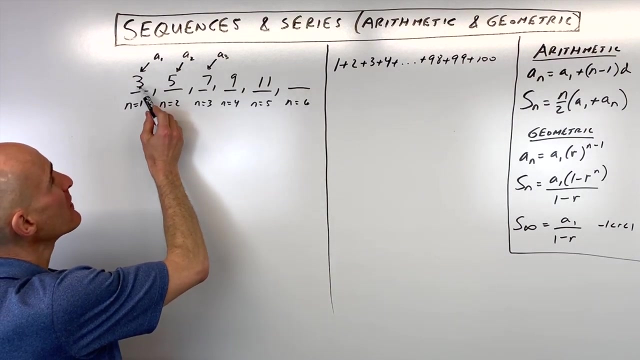 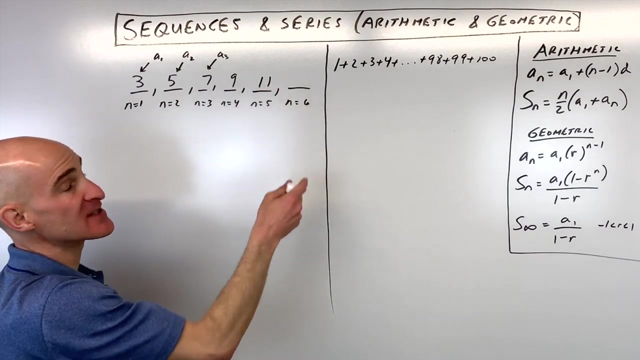 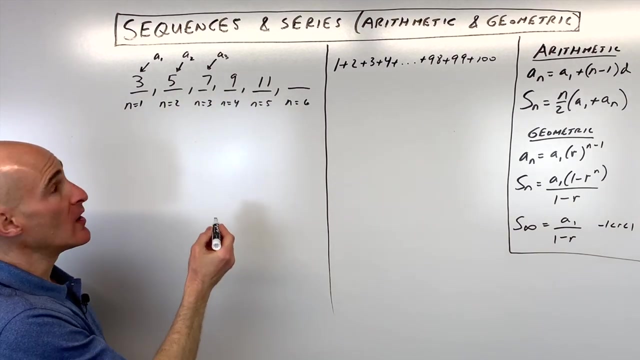 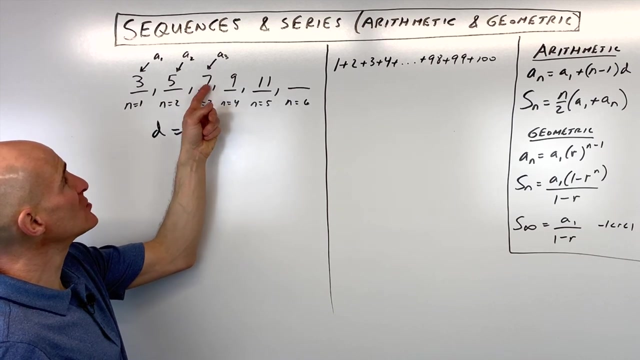 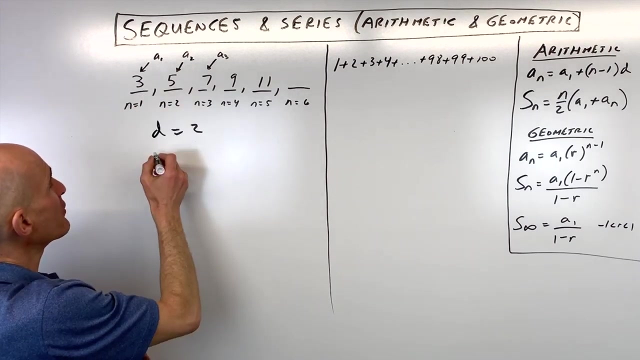 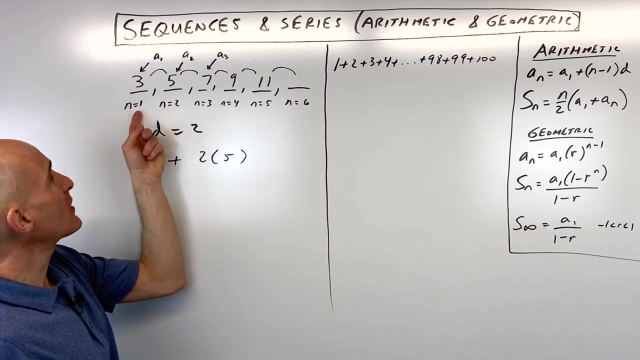